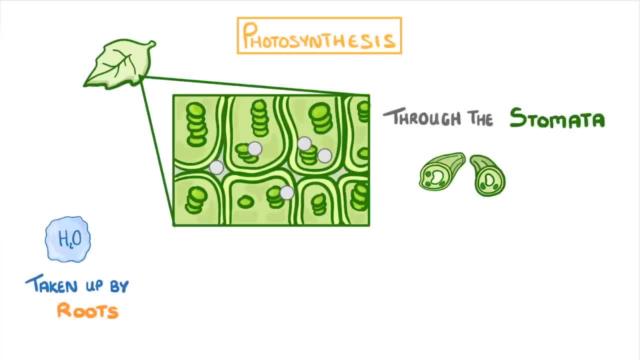 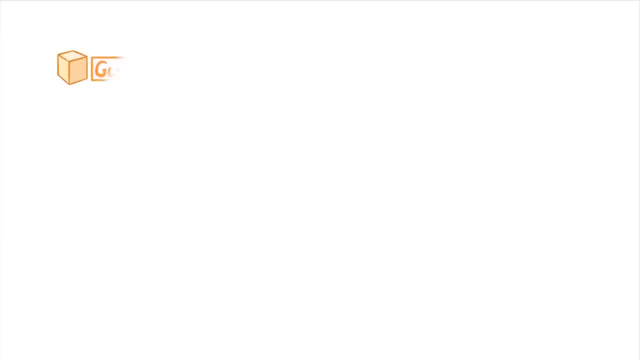 water is taken up from the soil by the roots and then transported to the leaves via the xylem. Now, the only product that the plants really want is the glucose. They do also sometimes use the oxygen for respiration, but there's so much oxygen in the air anyway that it's 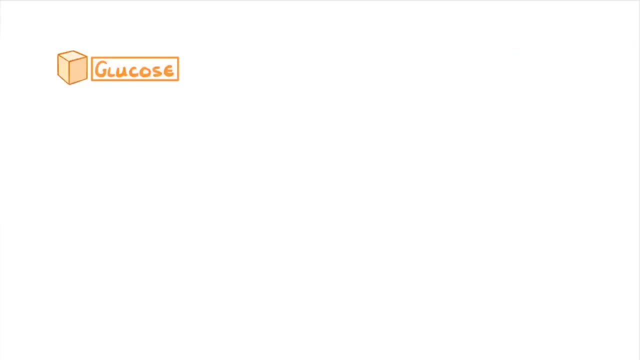 not too important. The glucose, though, is essential, and it's used mainly for 5 things. One is solar respiration, which breaks the glucose apart to release energy, So you can sort of think of glucose as a battery. Photosynthesis traps the sun's light energy in glucose molecules and then other cells around the. 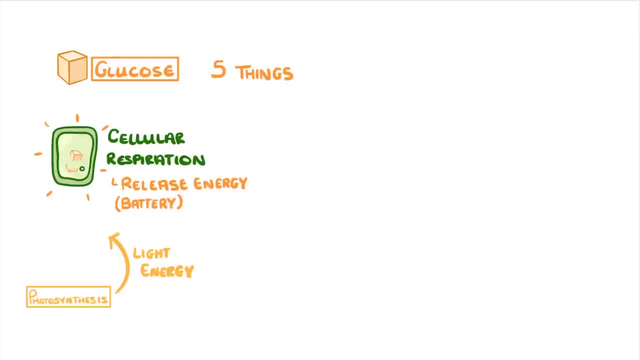 plant can break the glucose apart again to release that energy when they need it. The other four uses all involve making something out of glucose. For example, lots of glucose molecules can be combined to make cellulose, which is a complex carbohydrate that plants use to strengthen their cell walls. Glucose molecules can also combine to make starch. 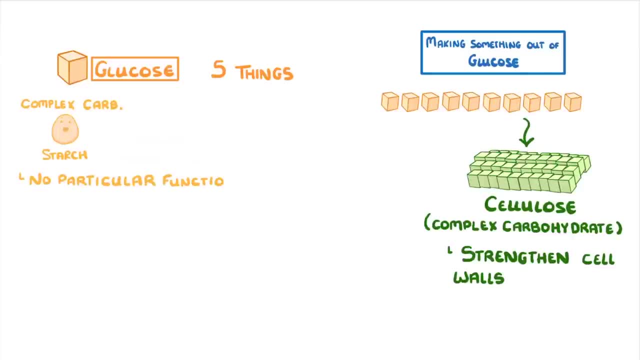 which is another complex carbohydrate, but it doesn't have a function as such. It's just a better form of glucose for long-term storage, because it's more compact, so you can fit a lot more of it within a cell and it's insoluble, which means that it won't. 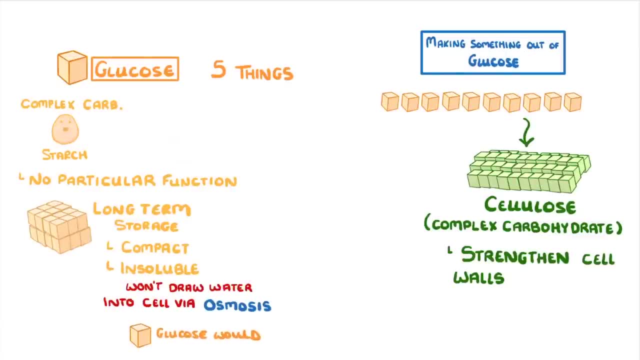 draw water into the cell through osmosis. like glucose would. Most plant cells try to keep a good store of starch so that they can break it down to glucose later, at times when photosynthesis isn't happening so much, for example during. 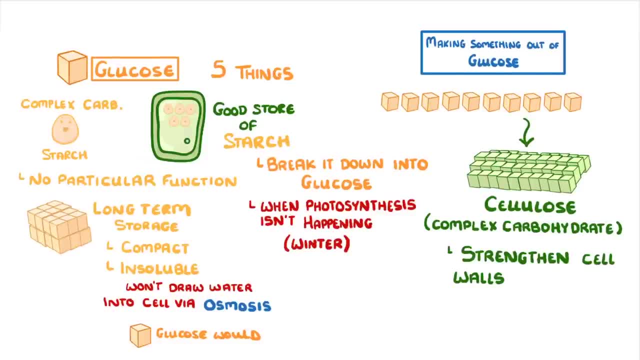 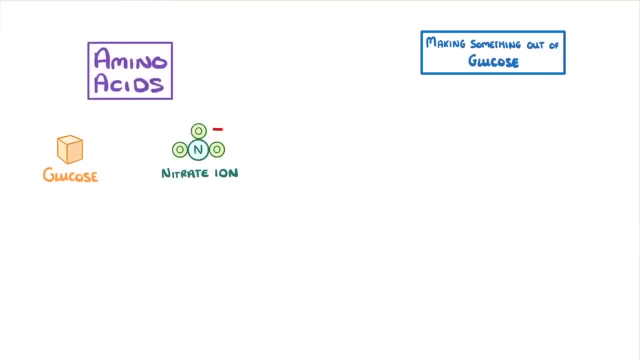 the night or in the winter. Another use is making amino acids, which they can do by combining the glucose molecules with nitrate ions which they get from the soil, And they can then combine these amino acids to make proteins. The final use is making oils and fats, which can also be stored as a future energy resource. 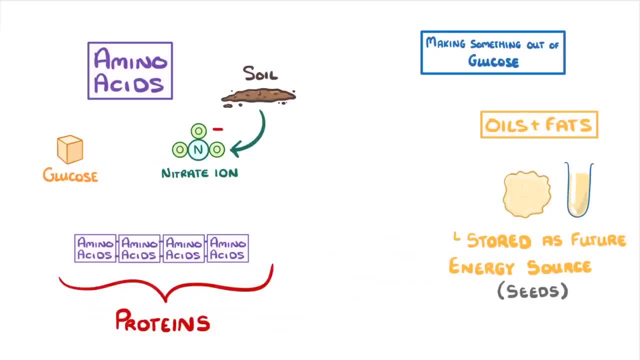 particularly for seeds, Because glucose is so essential for plants. their growth rate is often dependent on how fast they can produce glucose. This is because glucose is so essential for plants. their growth rate is often dependent on how fast they can produce glucose. So in the next video we'll explore the factors that affect the rate of photosynthesis. 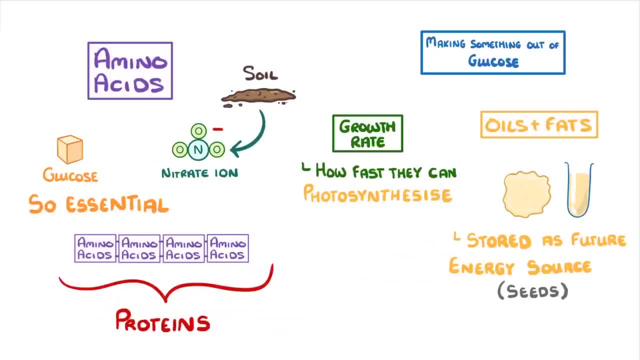 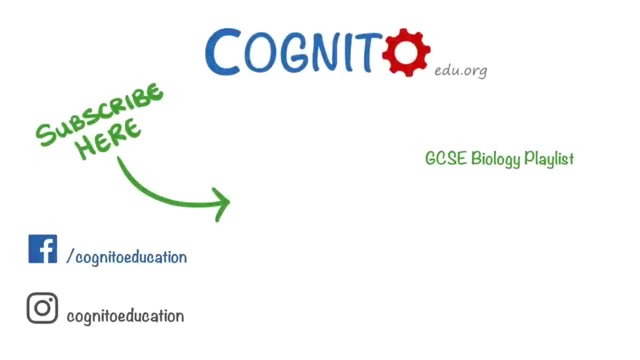 which are light intensity, temperature, carbon dioxide concentration and the amount of chlorophyll. That's everything for this video, though, so I hope you enjoyed it and we'll see you next time. 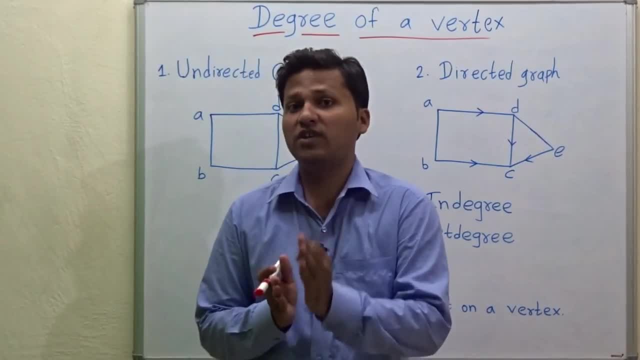 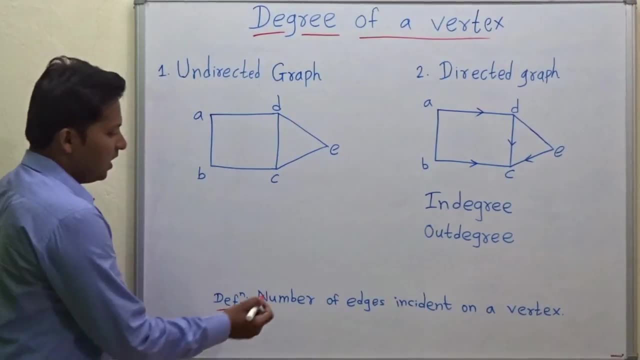 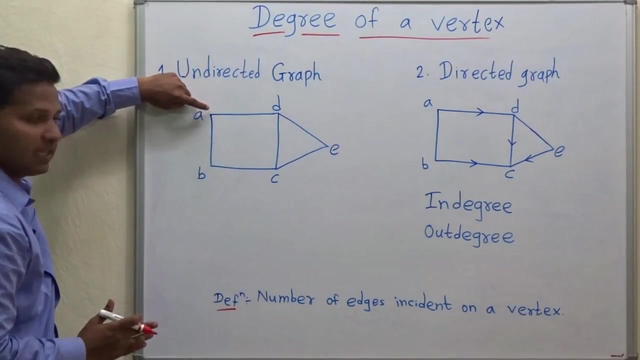 Hello friends, now we are going to see what is the degree of a vertex in graph. So let us see See. the definition for degree of a vertex is here. It is the number of edges incident on a vertex. That means, suppose this is a vertex A, So how many number of edges are incident on this? 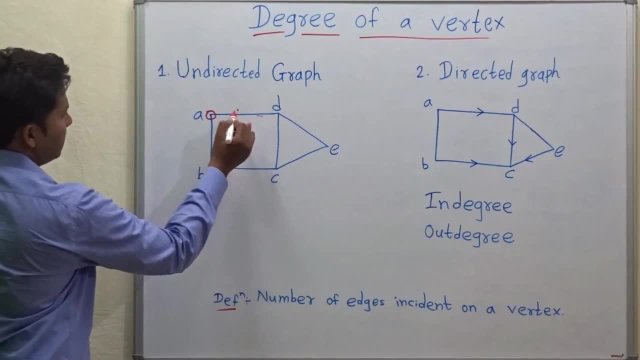 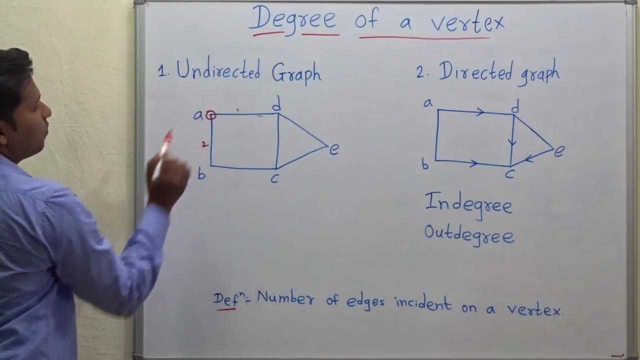 vertex. See, this is one edge, this one and this is the second edge. So these two edges are connected to this vertex means incident on this vertex. So these number of edges incident on this vertex or connected to this vertex is called as the degree of that vertex. So see what is. 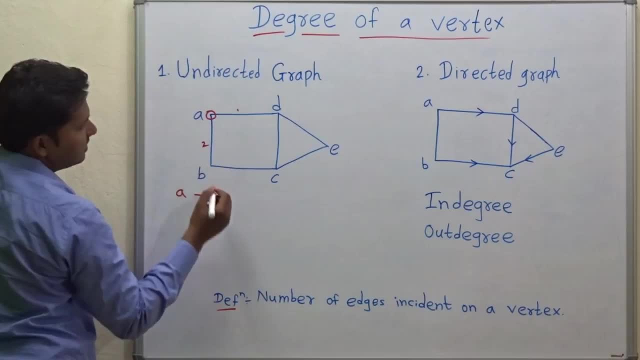 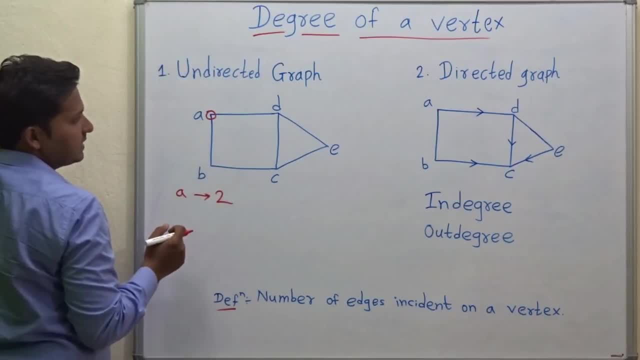 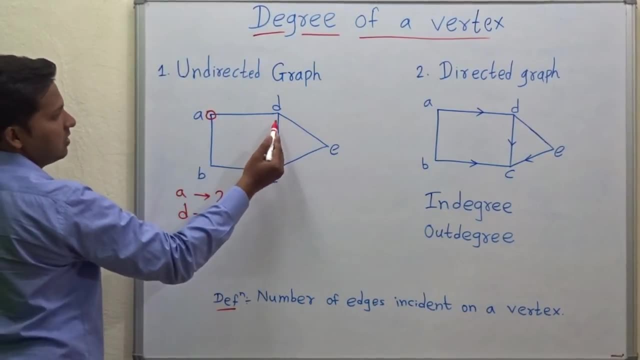 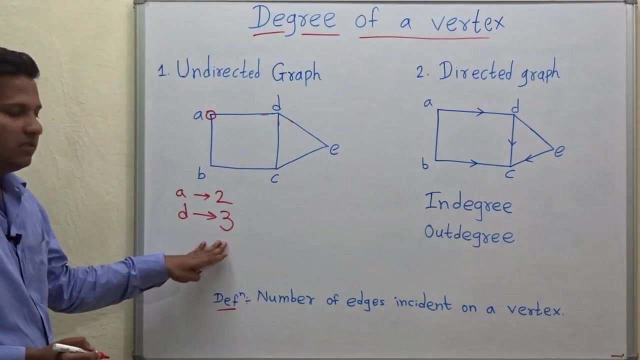 vertex. Now what is the degree of vertex D? See how many edges are connected to D or incident on D, See 1,, 2 and 3.. So the degree of vertex D is 3, right, Suppose if there is a vertex. 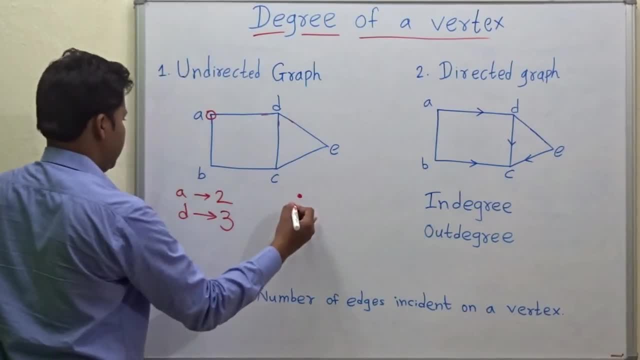 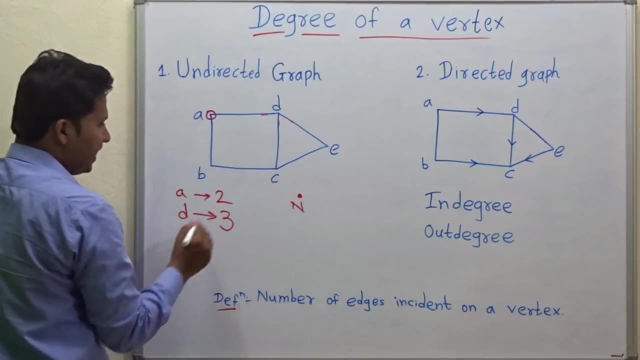 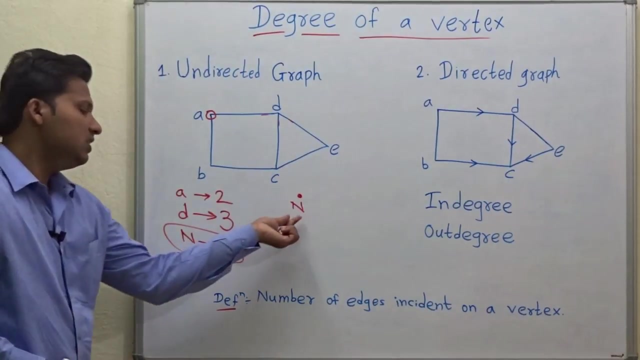 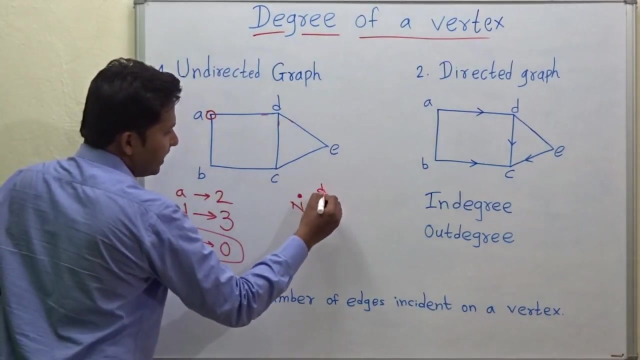 for which there is no edge connected. okay, If the vertex name is N and there is nothing connected to this vertex, then degree of vertex N will be 0,. okay, So the vertex which is not connected to any edge means the degree of that vertex is 0,. then that vertex is called as.